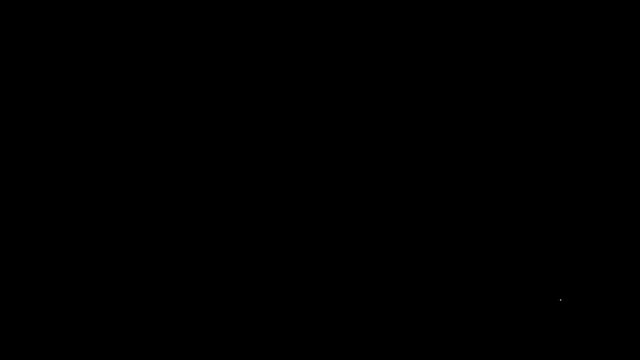 What is the difference between a monomial, a binomial, a trinomial and a polynomial? A monomial basically has one term. Example of monomials are 5x, 3,, 8x squared, 9x cubed. 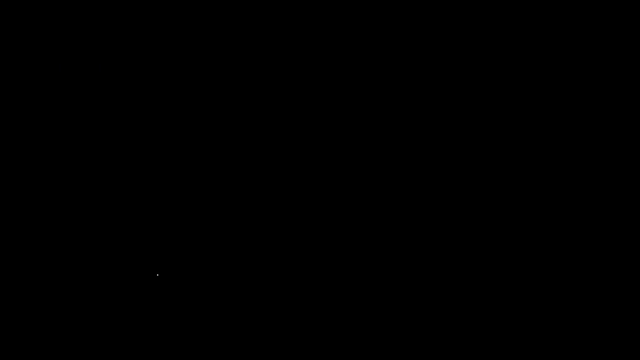 All of these are monomials. They have a single term. Mono means one, Bi means two, So a binomial is an expression that has two terms. So, for instance, x plus 5 is a binomial. x squared minus 3x, that's a binomial. x to the third plus 8, that's another one. 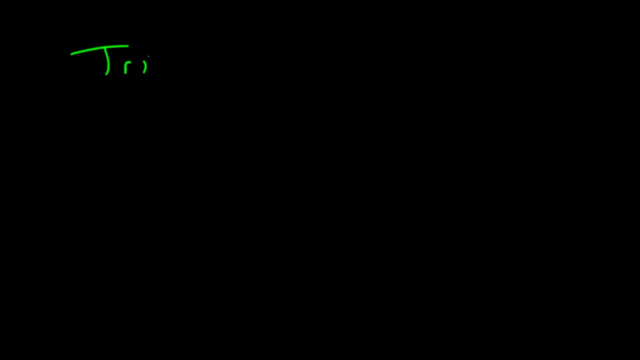 A trinomial has three terms. So an example of a trinomial would be x squared plus 5x minus 8.. Another example: x cubed plus 6x minus 7.. They all have three terms. A polynomial is an expression that simply has many terms. 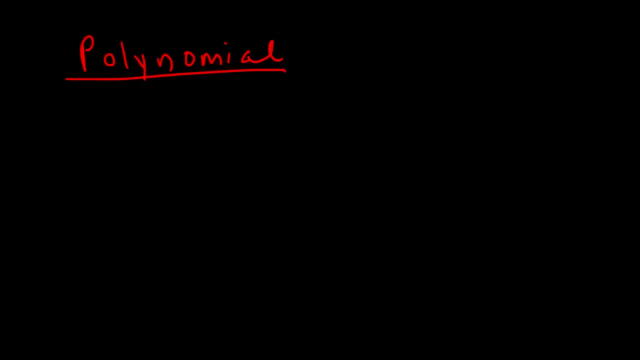 Poly means many 5x minus 7 plus x cubed. that's a polynomial. It's also a trinomial, but it can be classified as a polynomial: 9x to the fourth minus 5x plus 6x squared minus 7, that's a polynomial. 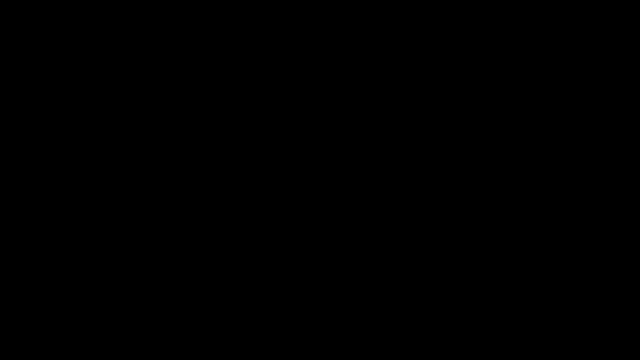 It has many terms. Now let's work on some examples. Go ahead and classify the following expressions as a monomial, binomial and trinomial, trinomial or polynomial. So let's start with the first one. Notice that we have three terms. 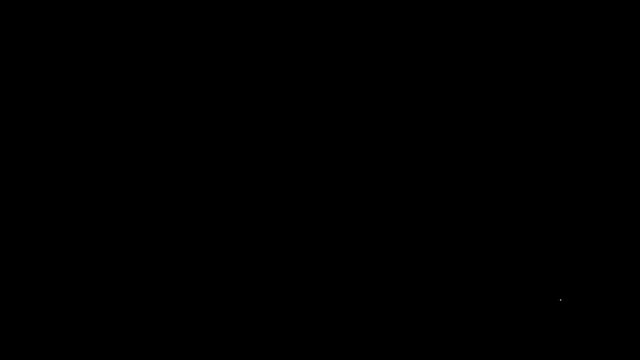 What is the difference between a monomial, a binomial, a trinomial and a polynomial? A monomial basically has one term. Example of monomials are 5x, 3,, 8x squared, 9x cubed. 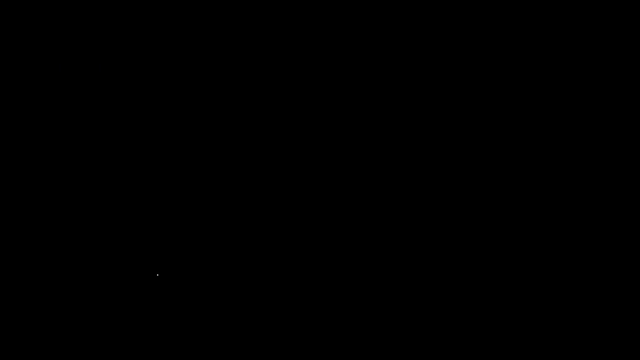 All of these are monomials. They have a single term. Mono means one, Bi means two, So a binomial is an expression that has two terms. So, for instance, x plus 5 is a binomial. x squared minus 3x, that's a binomial. x to the third plus 8, that's another one. 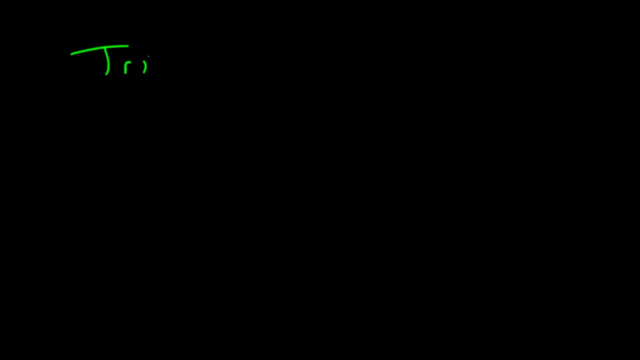 A trinomial has three terms. So an example of a trinomial would be x squared plus 5x minus 8.. Another example: x cubed plus 6x minus 7.. They all have three terms. A polynomial is an expression that simply has many terms. 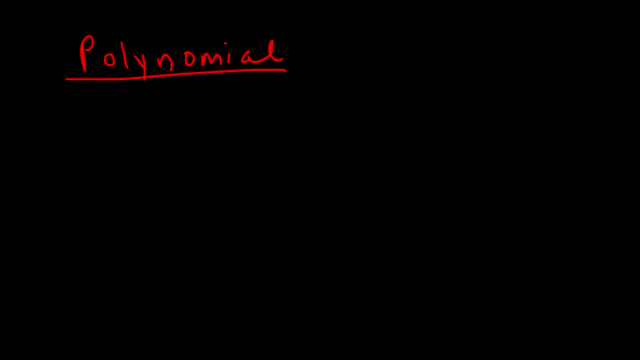 Poly means many: 5x minus 7 plus x cubed. that's a polynomial. It's also a trinomial, but it can be classified as a polynomial: 9x to the fourth minus 5x plus 6x squared minus 7, that's a polynomial. It has many terms. 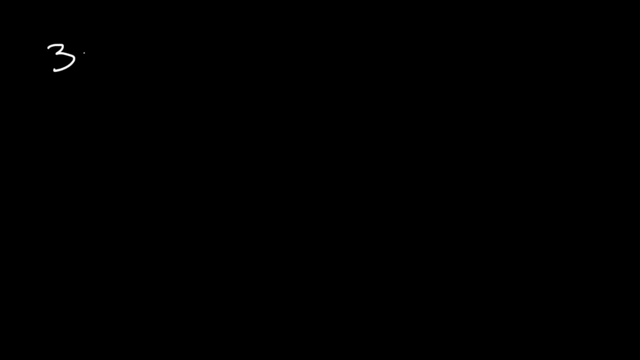 Now let's work on some examples. Go ahead and classify the following expressions as a monomial, binomial and trinomial, Trinomial, Trinomial or Polynomial. So let's start with the first one. Notice that we have three terms. 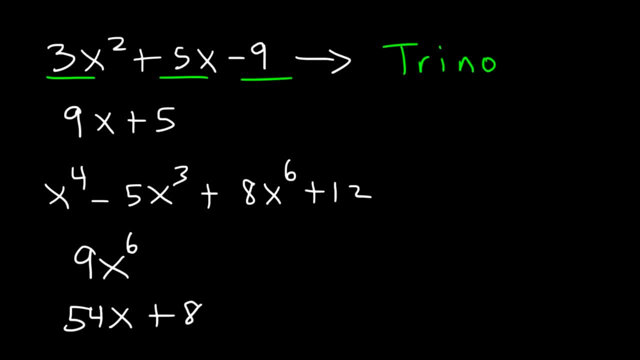 Therefore, this is classified as a Trinomial. Now, the second one only contains two terms, and two is associated with the word Bi, So this is going to be classified as a Binomial. Now, if it has more than three terms, like in this example, we have four terms simply. 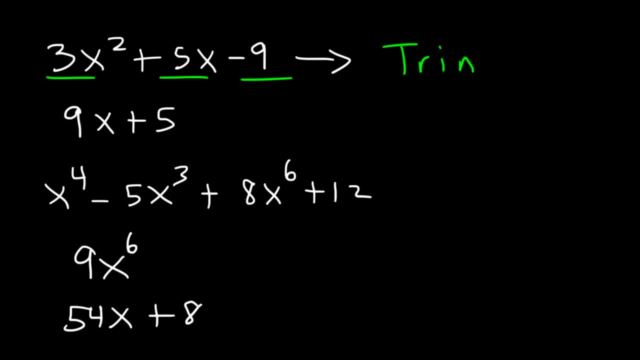 Therefore, this is classified as a trinomial. Now, the second one only contains two terms, and two is associated with the word by, So this is going to be classified as a binomial. Now, if it has more than three terms, like in this example, we have four terms. 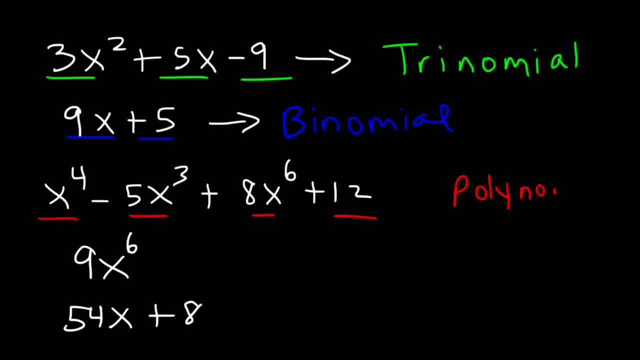 simply use the word polynomial. The next one only has a single term, so this is going to be called A monomial, And the last one has two terms, so it's a binomial. In this lesson, we're going to talk about how to identify the coefficients of every term. 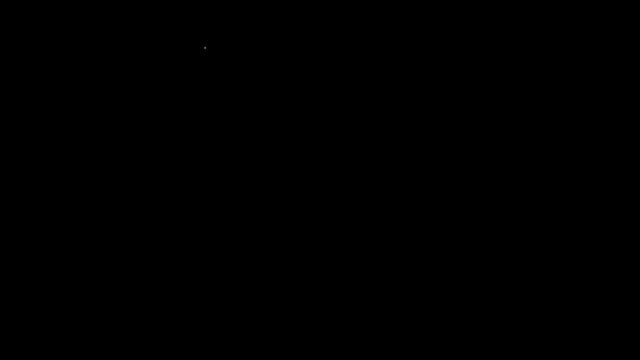 and also the degree of the polynomial. So let's say we have a polynomial that looks like this: 6x to the fourth, minus 5x, squared Plus 7.. So what are the terms in the polynomial? The terms are basically what you see. 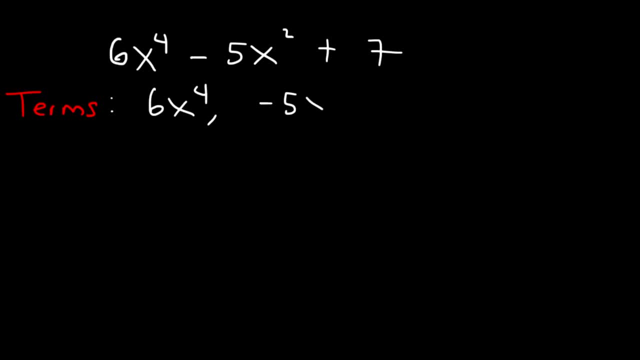 6x to the fourth is a term. Negative, 5x squared is a term And 7 is a term. Now, what are the coefficients of every term in this expression? The coefficient of the first term, which is 6x to the fourth. 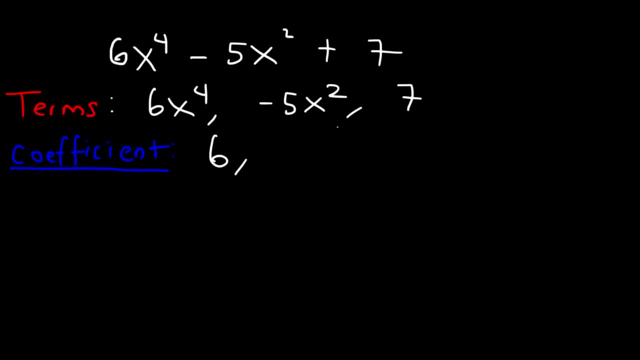 is the number in front of x, It's 6.. The coefficient of the second term is negative: 5.. And the coefficient of the last one is 7.. Now what is the degree of each term in this expression? The degree of the first term is basically the exponent that you see. 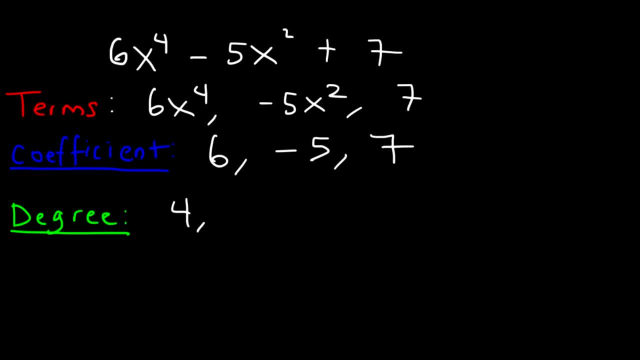 It's 4.. The degree of the second term is 2.. The degree of a constant. there's no x value next to it, so it's going to be 0.. Now, what is the lead-in term And also what is the lead-in coefficient? 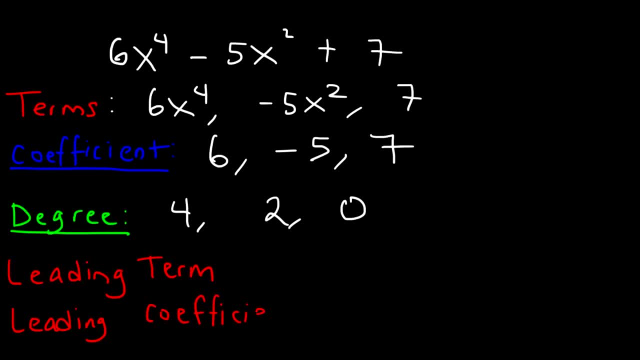 What do you think the answer to those questions are: The lead-in term is the term with the highest degree. So it's 6x to the fourth: The lead-in coefficient is the term with the highest degree. The lead-in coefficient is simply the coefficient of the lead-in term. 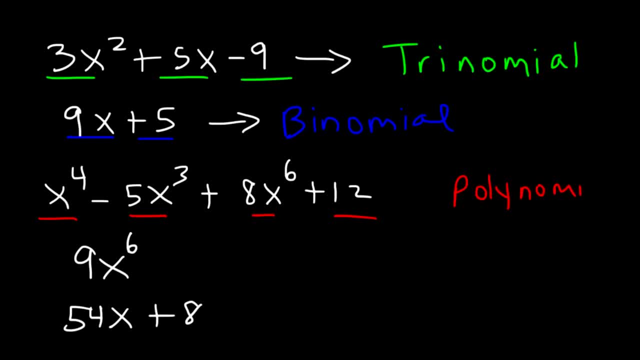 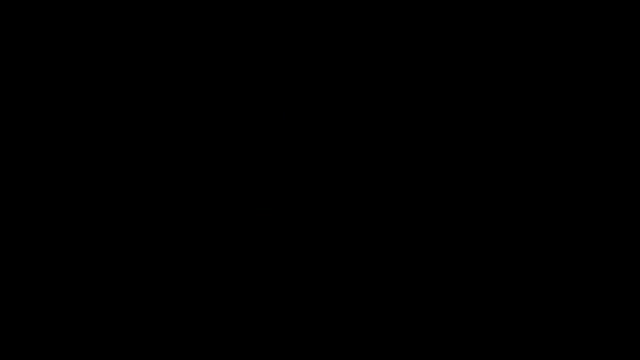 use the word Polynomial. The next one only has a single term, So this is gonna be called a Monomial, And the last one has two terms, so it's a Binomial. In this lesson we're going to talk about how to identify the coefficients of every term. 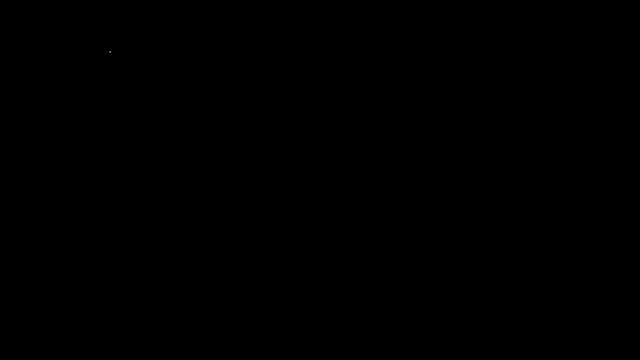 and also the degree of the polynomial. So lets say, if we have a polynomial looks like this: 6x to the fourth, minus 5x squared plus 7. so what are the terms in the polynomial? the terms are basically what you see: 6x to the fourth. 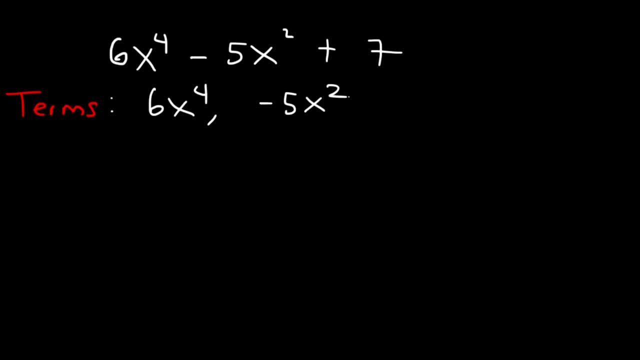 is a term, negative, 5x squared is a term and 7 is a term. now, what are the coefficients of every term in this expression? the coefficient of the first term, which is 6x, to the fourth, is the number in front of X: it's 6. the 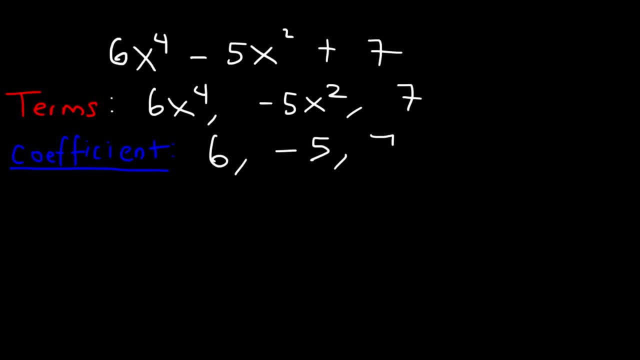 coefficient of the second term is negative, 5, and the coefficient of the last one is 7. now what is the degree of each term in this expression? the degree of the first term is basically the exponent that you see, it's 4. the degree of the second term is 2, the degree of a constant. there's no X value. 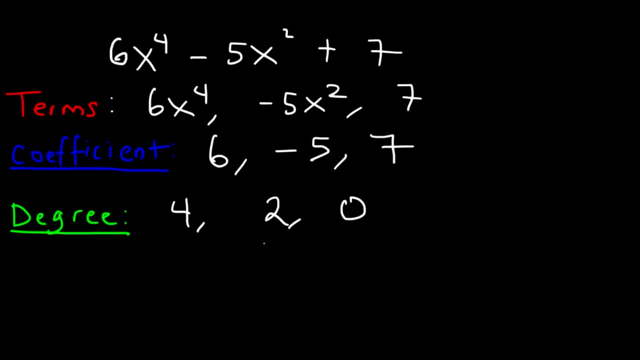 next to it. so it's going to be 0. now, what is the lead-in term? and also, what is the lead-in coefficient? what do you think? the answer to those questions are you? the lead-in term is the term with the highest degree, so it's 6x to the fourth. 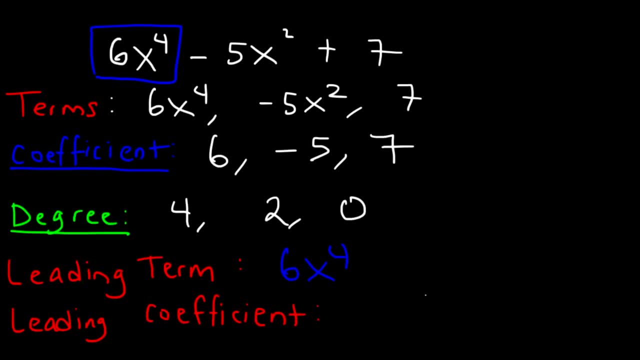 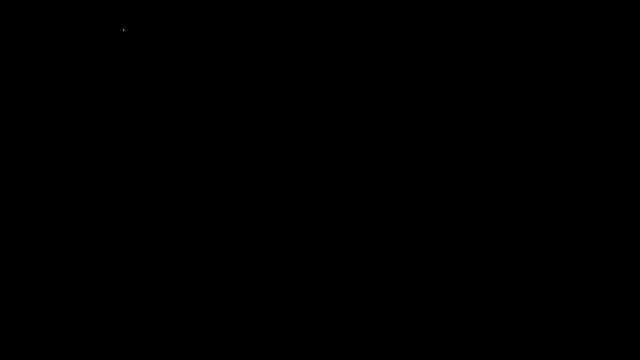 the leading coefficient is simply the coefficient of the leading term. it's 6. now what is the degree of the entire polynomial? the degree of the polynomial is basically the highest of these numbers, so it's degree 4. now let's work on another example. so let's say, if we have a polynomial that 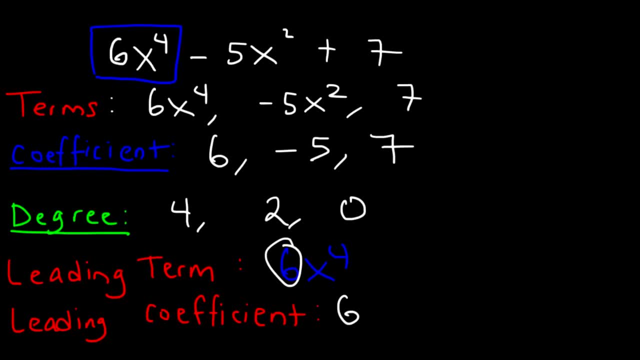 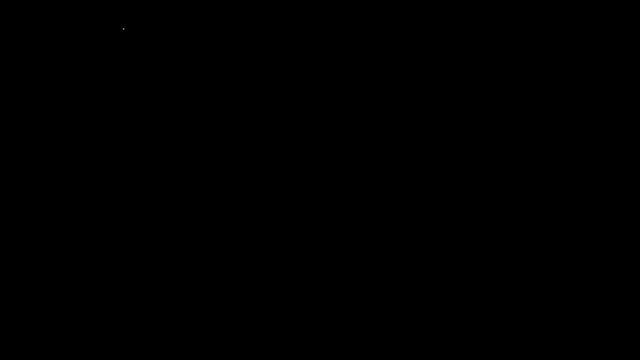 It's 6.. Now what is the degree of the entire polynomial? The degree of the polynomial is basically the highest of these numbers, So it's degree 4.. Now let's work on another example. So let's say if we have a polynomial that looks like this: 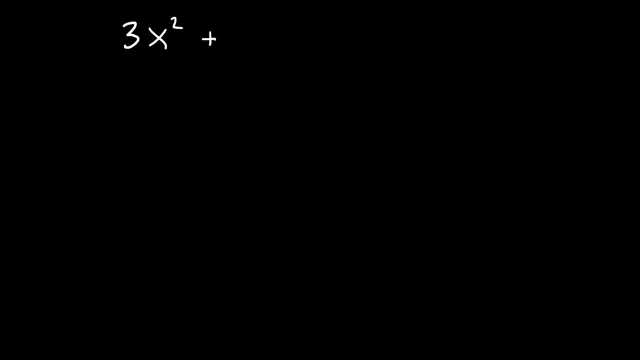 3x squared plus 8.. Minus 9x plus 7x to the fifth power. So, just like before, identify all of the terms in this particular polynomial expression, Identify the coefficient of every term And then, after that, identify the degree of each term. 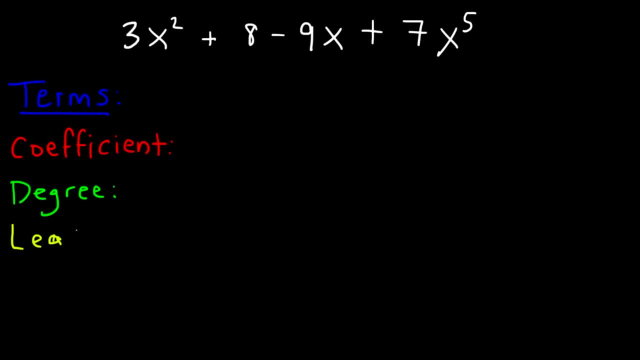 Next determine the lead-in term, The lead-in coefficient And finally, the degree of of the polynomial. So feel free to pause the video and work on this example. Go ahead and fill this in. So the terms are. let's list them in descendant order: 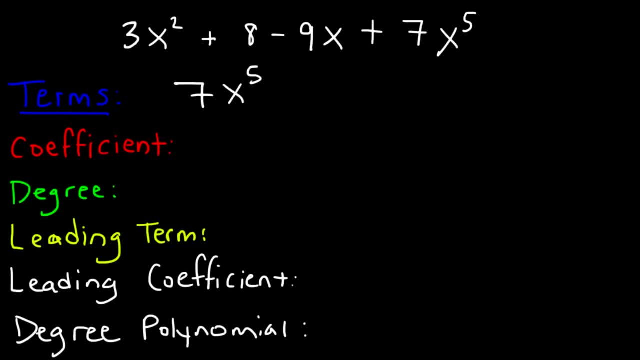 7x to the fifth, And then we have 3x squared Negative, 9x and eight. All of these are individual terms. The coefficient of each term is 7,, 3,, negative, 9, and 8.. Now the degree of each of those terms. the first one has a 5 as an exponent, so it's degree 5.. 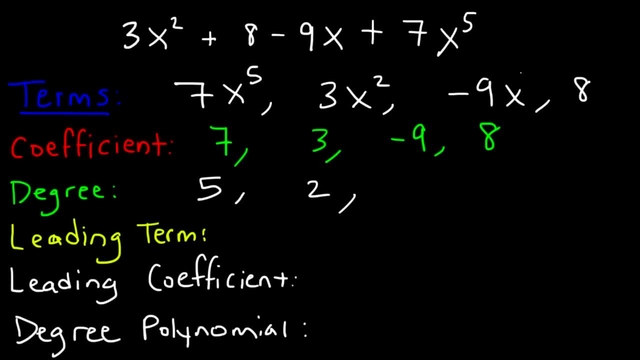 The second one is 2.. The next one: we have an invisible 1. And for the constant term it doesn't have a degree, It's degree 0.. Now, the lead-in term is 0.. It's basically the term with the highest degree. 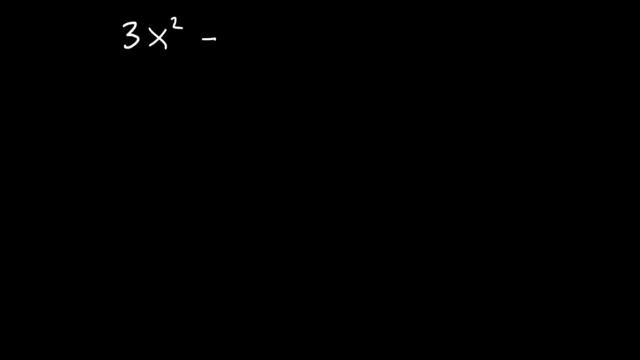 looks like this: 3x squared plus 8 minus 9x plus 7, x to the fifth power. so, just like before, identify all of the terms in this particular polynomial expression, identify the coefficient of every term and then, after that, identify the degree of each term. 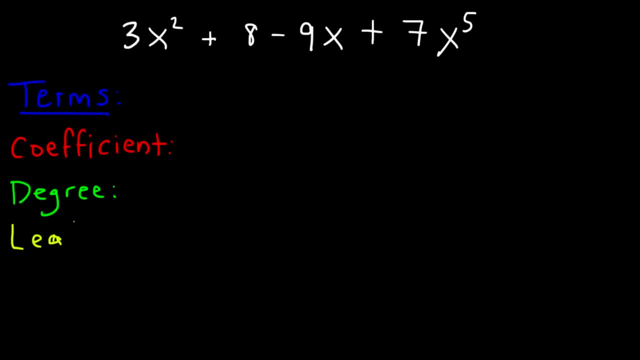 next determine the leading term, the leading coefficient and, finally, the degree of the polynomial. so feel free to pause the video and work on this example. go ahead and fill this in. so the terms are. let's list them in descendant order: 7x to the fifth. and then we have 3x squared. 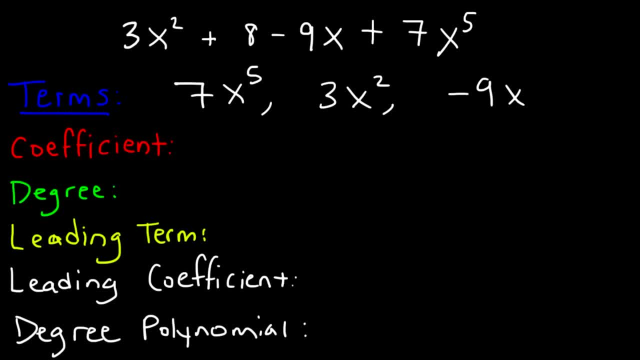 negative, 9x and 8. all of these are individual terms. the coefficient of each term is 7, 3 negative, 9 and 8. now the degree of each of those terms. the first one has 5 as an exponent, so it's degree 5. 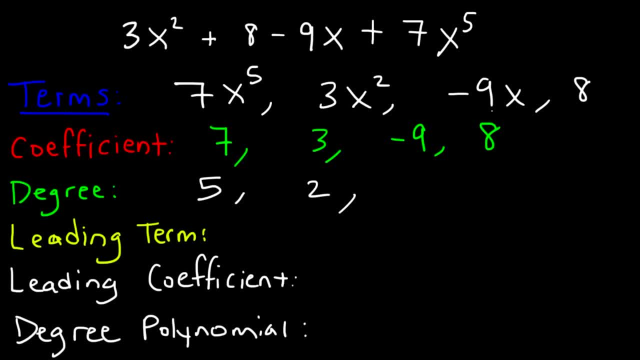 the second one is 2, the next one we have an invisible 1 and for the constant term it doesn't have a degree, it's degree 0. now the leading term is basically the term with the highest degree. it's not necessarily the first one. so the leading term is 7x to the fifth. 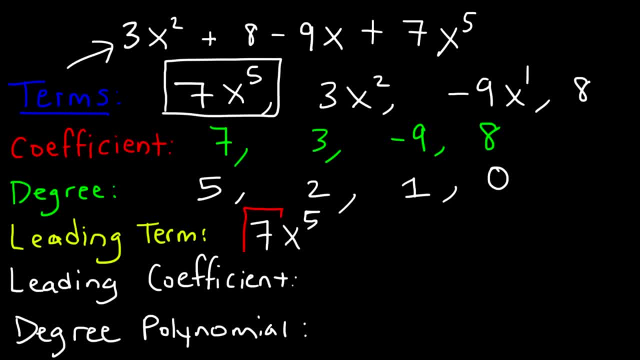 power. the leading coefficient is simply the number of that term, the number in front of the x. so the leading coefficient is 7x to the fifth power. the division of 7 and the degree of the entire polynomial is basically the degree of the leading term. so that's the highest degree, so it's 5. 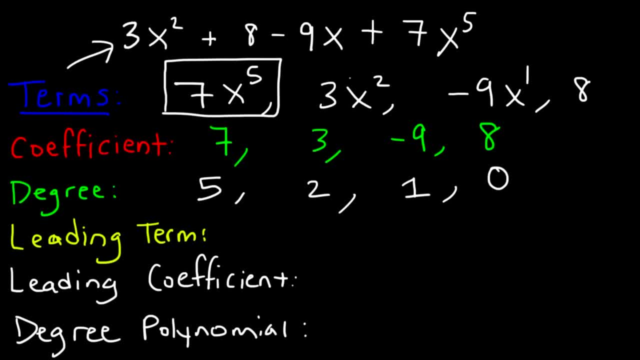 It's not necessarily the first one. So the lead-in term is 7x to the fifth power. The lead-in coefficient is simply the number of that term, The number in front of the x. So the lead-in coefficient is 7.. 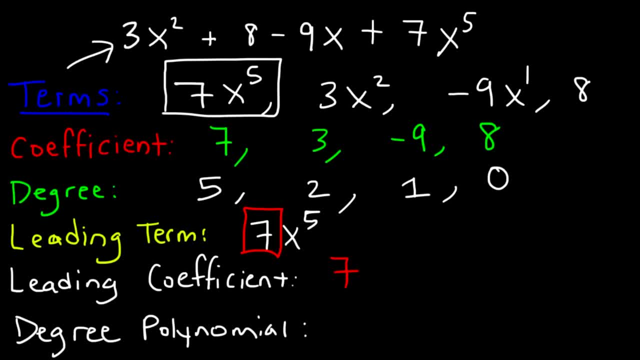 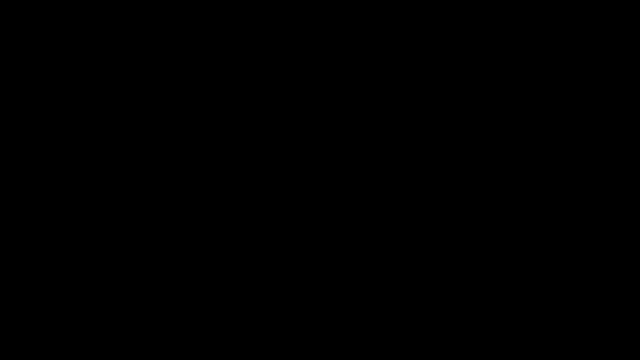 And the degree of the entire polynomial is basically the degree of the lead-in term. So that's the highest degree, So it's 5.. Now what if we have multiple variables? Let's say, if we have a polynomial expression that looks like this: 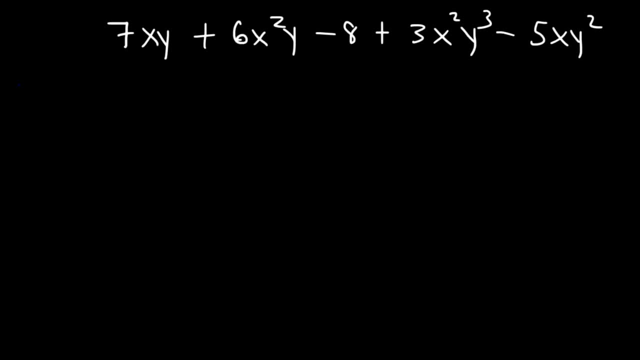 So go ahead and identify all of the terms, just like we did before, And then identify the coefficient And then identify the coefficient of each of those terms. Next, find the degree of those terms And then identify the lead-in term And then, after that, the lead-in coefficient. 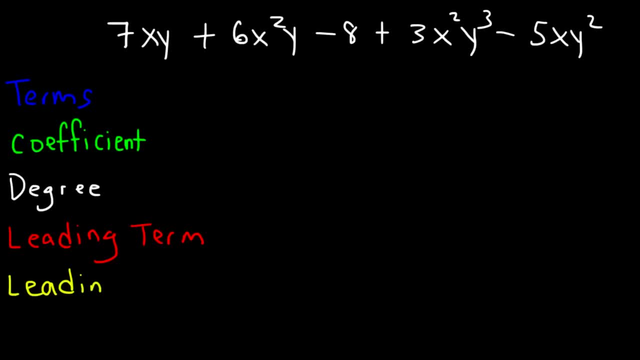 And then after that the lead-in coefficient And then finally the degree of the polynomial itself. So go ahead and try this. So let's identify all the terms And let's put it in descendant order. So the highest term is going to be 3x squared y cubed. 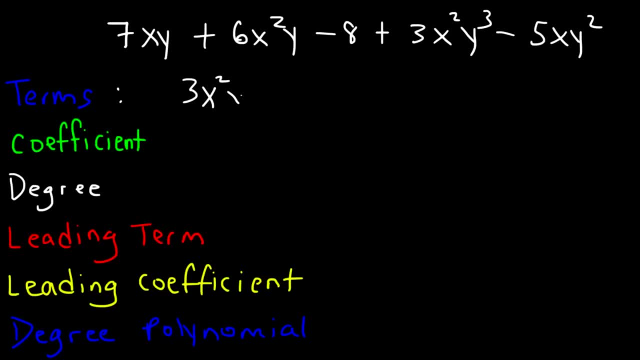 If you add up all the exponents, you're going to get the highest number. The next one is going to be well, 6x squared y and 5xy squared. The sum of the exponents are the same, It's 3.. 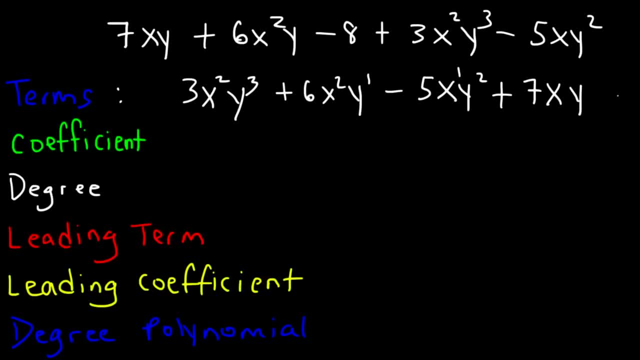 And then we have 7xy And finally negative 8.. So we have a total of 5 terms. Now the coefficients of each term are the same. The coefficients of each term are 3,, 6,, negative 5,, 7, and negative 8.. 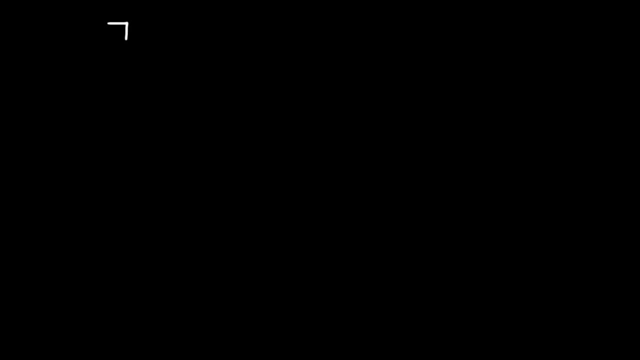 now what if we have multiple variables? let's say, if we have a polynomial expression that looks like this, with punctuation, let's focus on the Einstein intermediarius aagnbirds splice. so go ahead and identify all of the terms, just like we did before, and then identify the coefficient of each of those terms. next, find a degree of those. 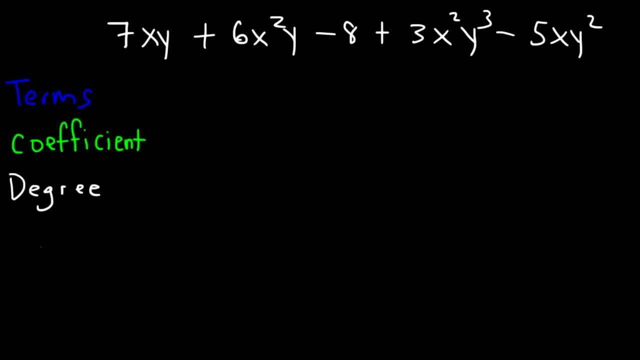 terms and then identify the leading term and then after that the lead-in coefficient and then finally, the degree of the polynomial itself. so go ahead and try this. so let's identify all the terms and let's put it in descending order. so the highest term is going to be 3x squared y cube, if you. 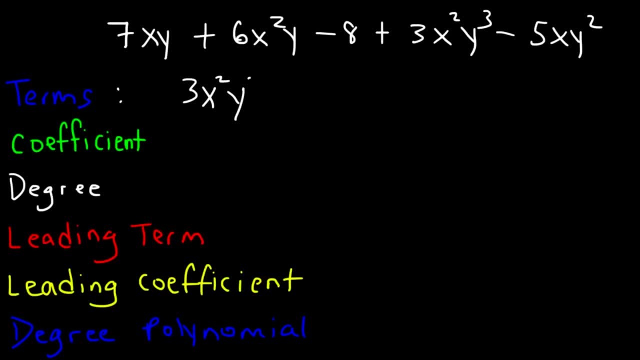 add up all the exponents, you're going to get the highest number. the next one is going to be well, 6x squared y and 5x y squared. the sum of the exponents are the same, it's 3. and then we have 7 x- y and 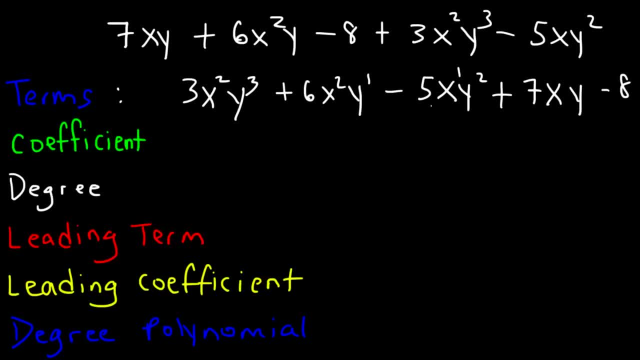 finally, negative 8. so we have a total of five terms. now the coefficients of each term are 3, 6, negative 5, 7 and negative 8. the degree of each term, the degree of the first one: just add the exponents: 2 plus 3 is 5. for the second one, 2 plus 1 is 3 for the. 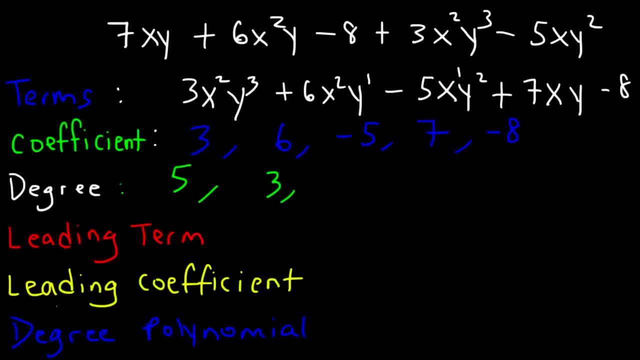 third one, 1 plus 2 is 3, and for the fourth one there's two invisible ones, which adds up to 2, and the last one is a constant and doesn't have a variable, so it's degree 0. the leading term is basically the one with the highest.